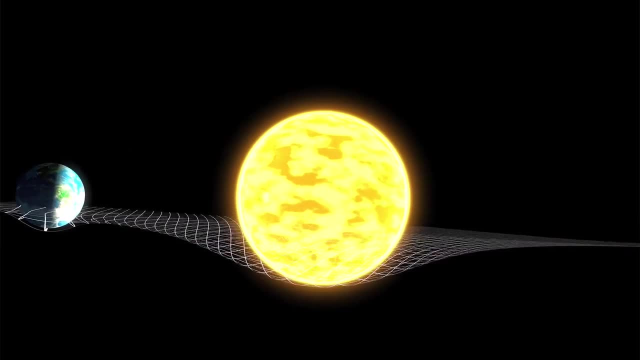 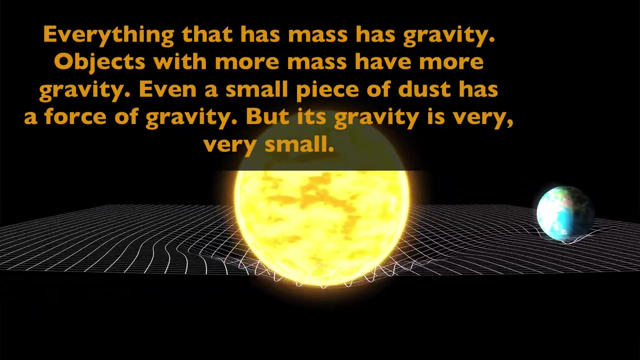 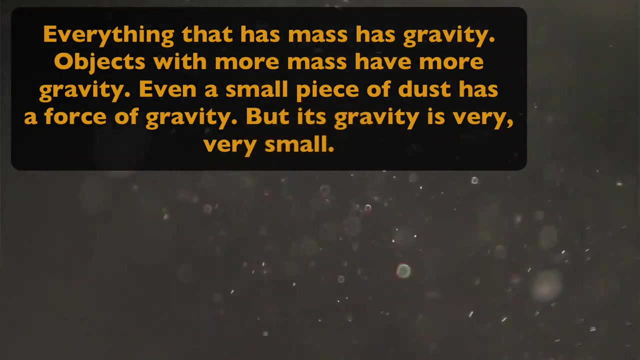 And this is known as the object's mass or mass. See, everything that has mass has gravity, So objects with more mass have more gravity. Even a tiny, small speck of dust has its own force of gravity, But its gravity is very, very small compared to something like a bowling ball. 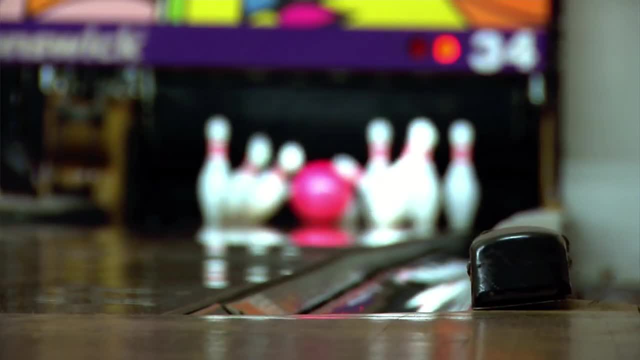 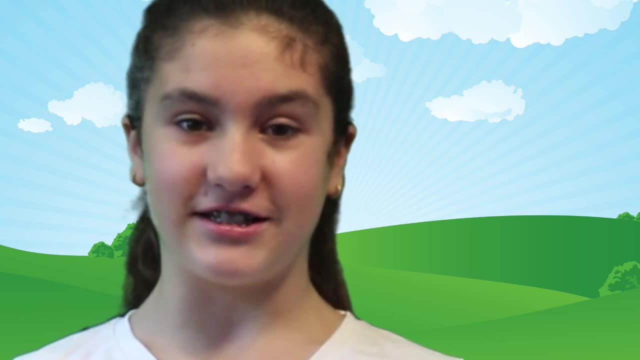 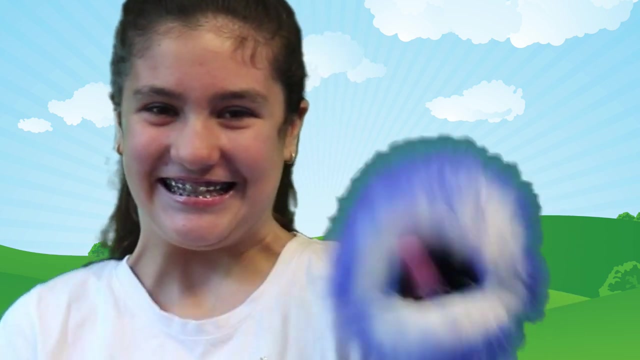 which is heavy and larger than a piece of dust. Because it's bigger and has more mass, it has more gravity. The closer these objects are to each other, the stronger their gravitational pull. is Gravitational. I think it's gravitational. 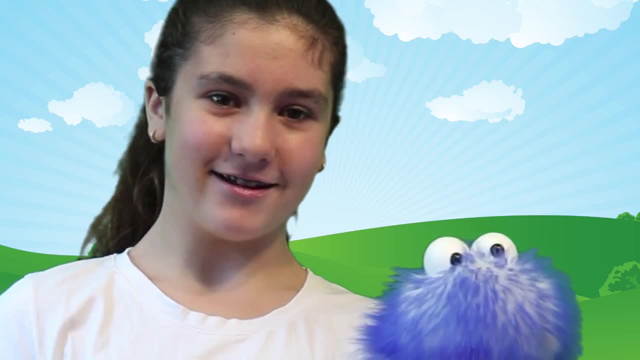 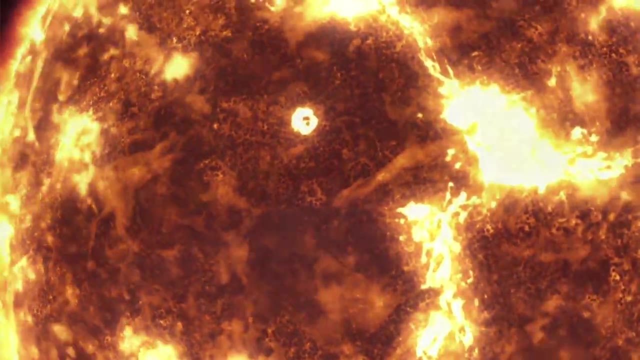 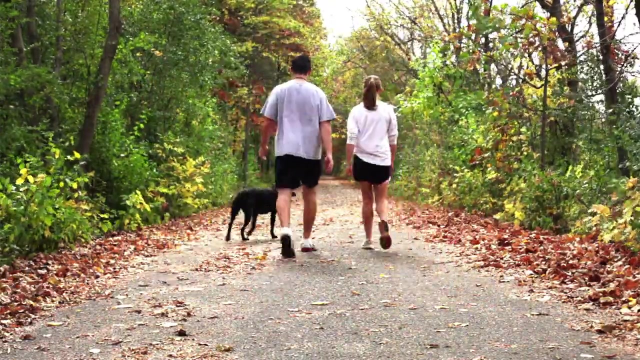 Oh, my bad. Yeah, you are bad. For example, the Sun has a lot more gravity than our planet, the planet Earth, But we stay on Earth's surface and don't get pulled to the Sun because we live here. We're much closer to the Earth than the Sun. 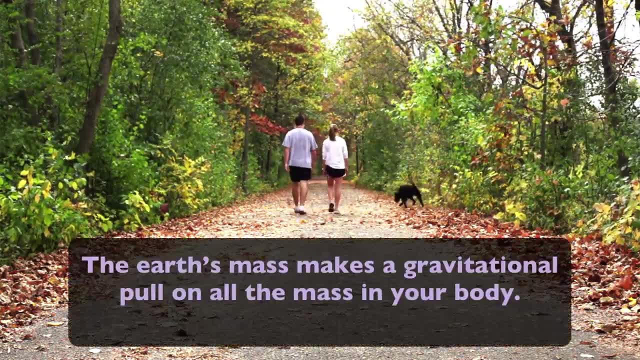 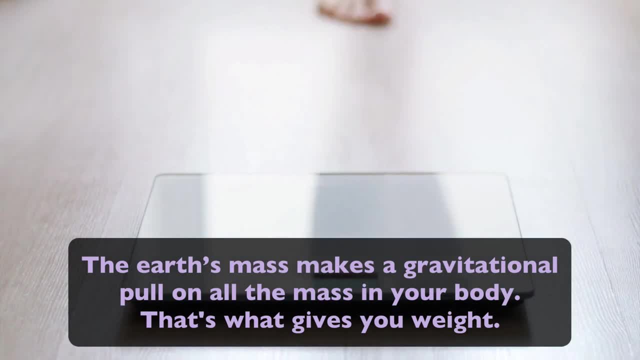 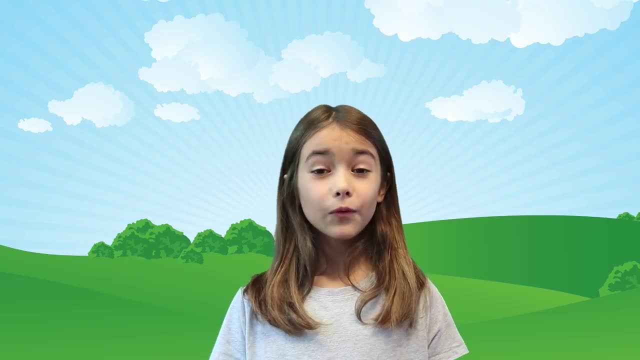 And the Earth's mass makes a gravitational pull on the mass in your body And, believe it or not, that's what gives you weight, And we'll learn more about that in a few more minutes. Stay tuned. The force of gravity keeps all of the plants in orbit around the Sun. 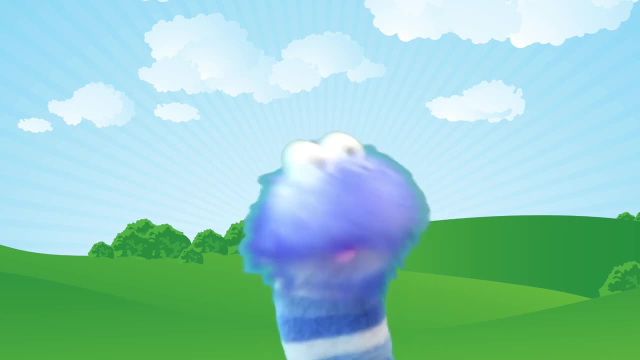 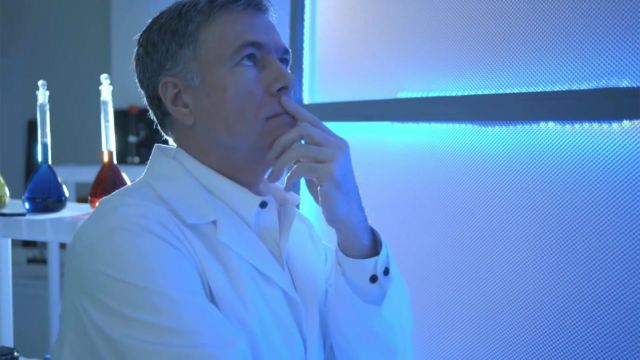 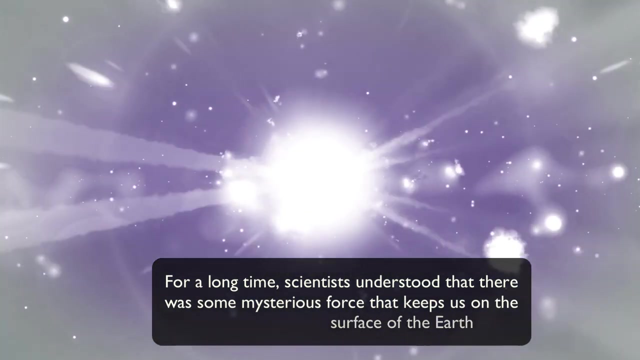 Well, I definitely know it wasn't me. So who discovered gravity? That's actually a really good question, Gus See. for a long time scientists understood that there was some mysterious force that keeps us on the surface of the Earth. 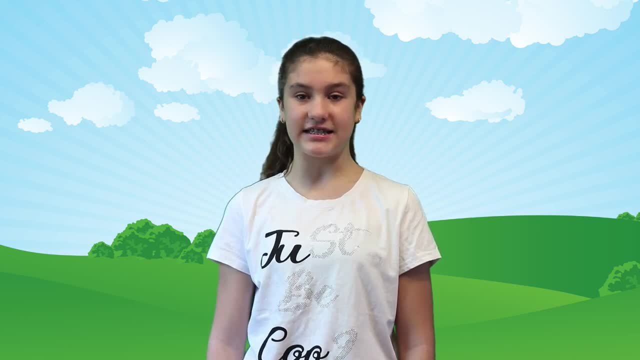 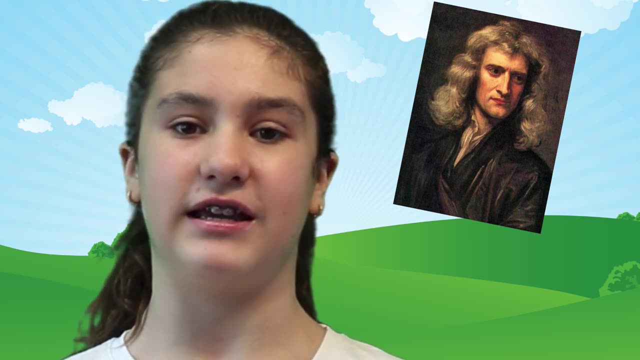 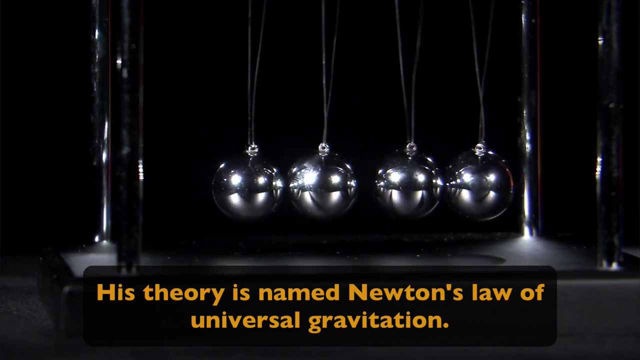 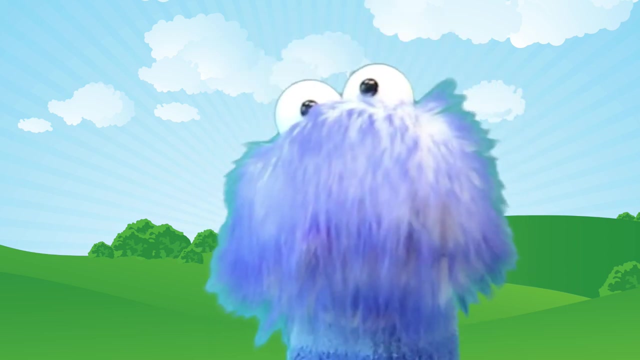 But it wasn't until 1666 that Isaac Newton first described his theory on the force of gravity, And his theory is called Newton's Law of Universal Gravitation. It is said that his ideas about gravity were inspired by watching an apple fall from a tree. 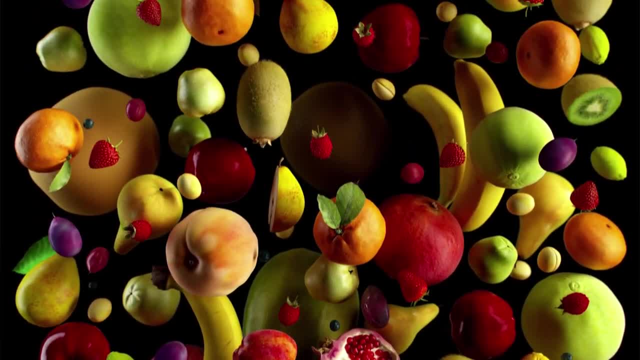 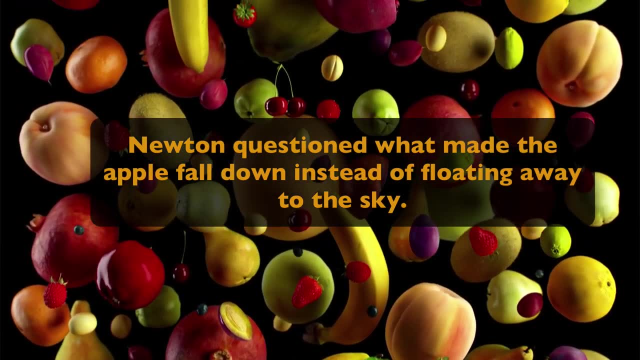 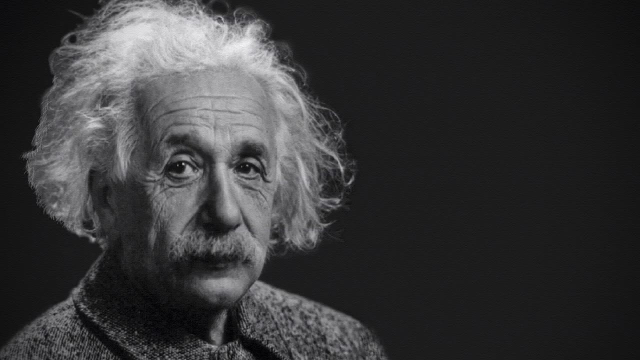 Hmm, You see, Isaac Newton saw something very familiar. He saw an apple fall down and questioned and thought: what made the apple fall down instead of floating away to the sky? Then Albert Einstein, another famous scientist that you've probably heard of. 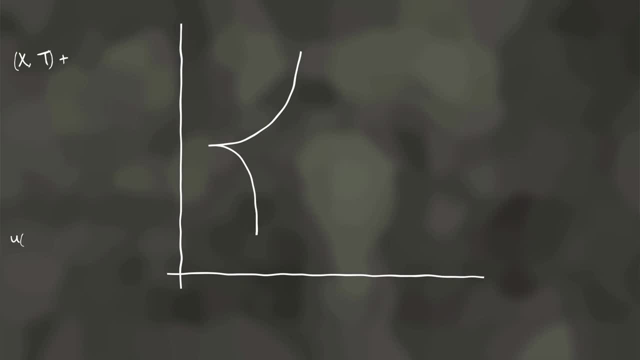 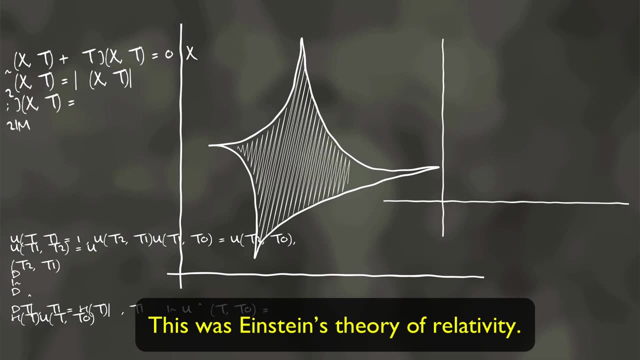 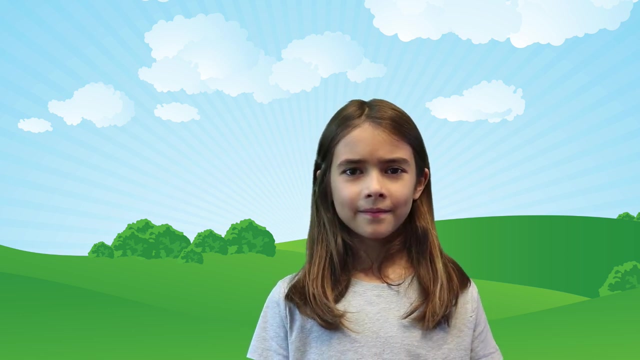 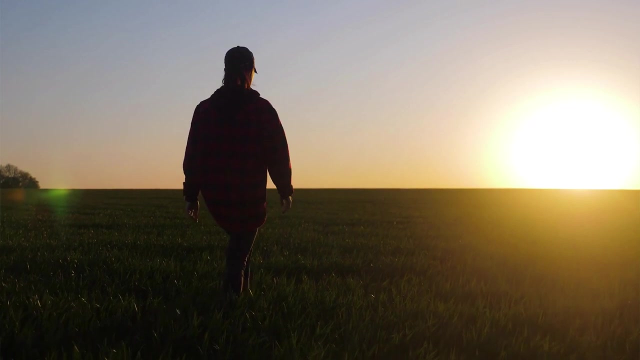 later made some improvements on Newton's theory, And when he made this improvement, this was called Einstein's Theory of Relativity. So why is gravity important? Well, like we talked about before Quinn, without Earth's gravity we would float right off of our planet. We'd float right off of Earth into space. So we'd all have to be glued down all the time And forget about it. If you kicked or threw a ball, like we do in the backyard sometimes, it would float away forever. Hey, guess what? 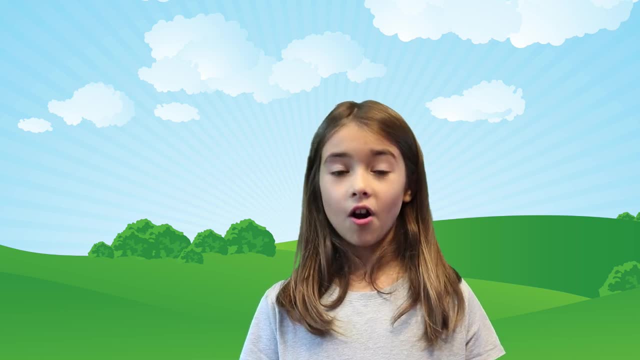 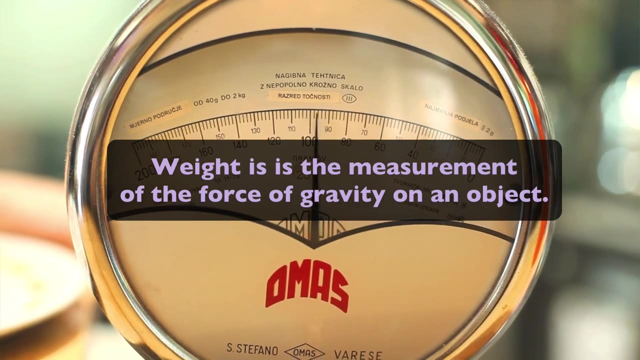 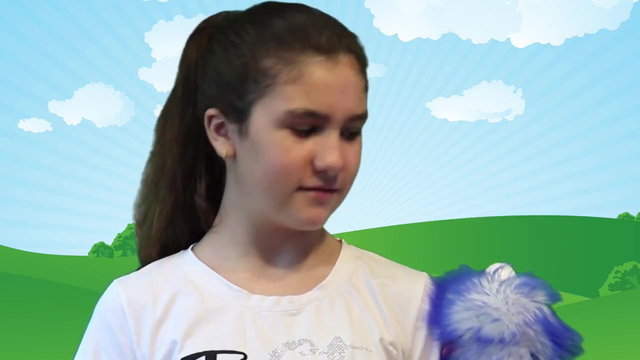 Did you know that weight is based on gravity? That's right. Weight is the measurement of the force of gravity on an object. This means your weight is how hard gravity is pulling you toward the Earth's surface. Gus, what are you doing? 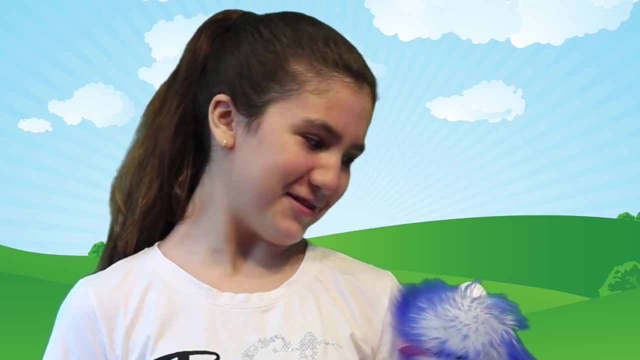 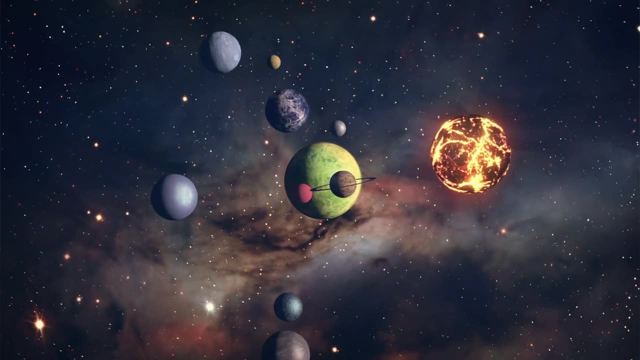 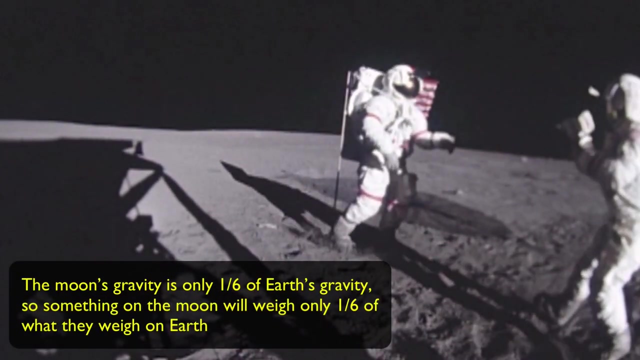 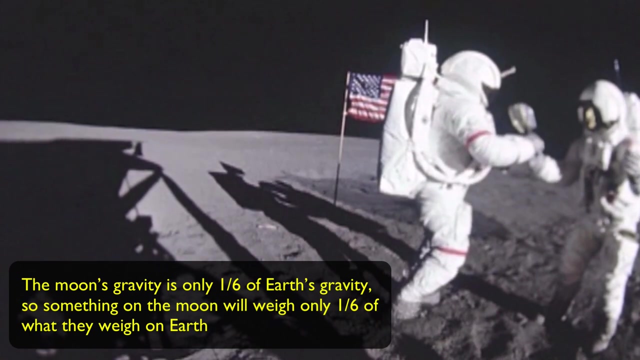 Trying to beat gravity and pulling it down. It's not working. You would actually weigh less on smaller planets and even more on larger planets. For example, the Moon's gravity is only one-sixth of Earth's gravity, So something on the Moon will weigh only one-sixth of what they weigh on Earth. 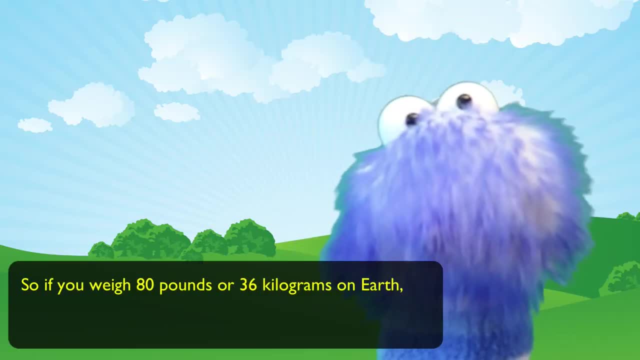 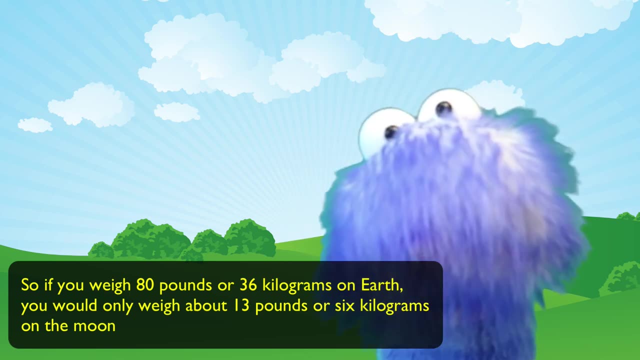 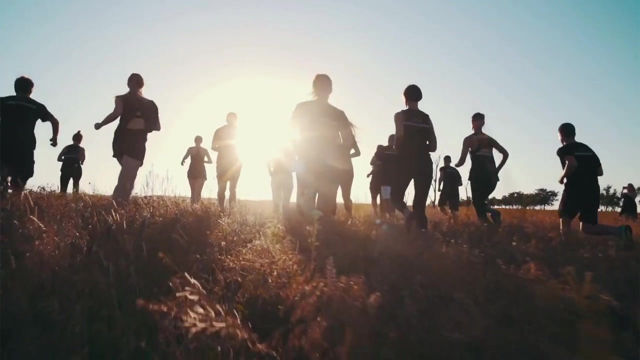 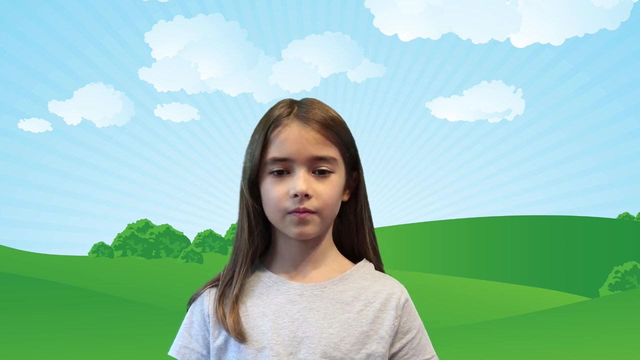 So if you weigh 80 pounds or 36 kilograms on Earth, you would only weigh about 13 pounds or 6 kilograms on the Moon. Gravity is very important to our everyday lives, But gravity also is important for much bigger reasons too. 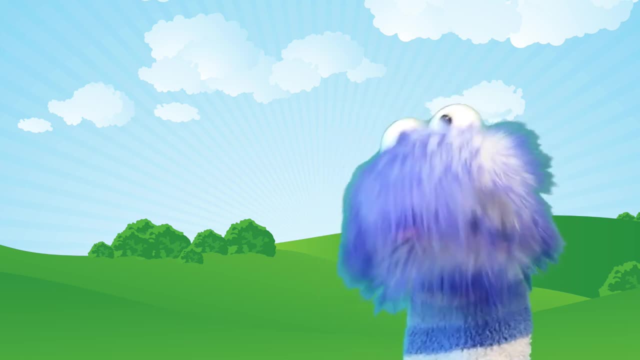 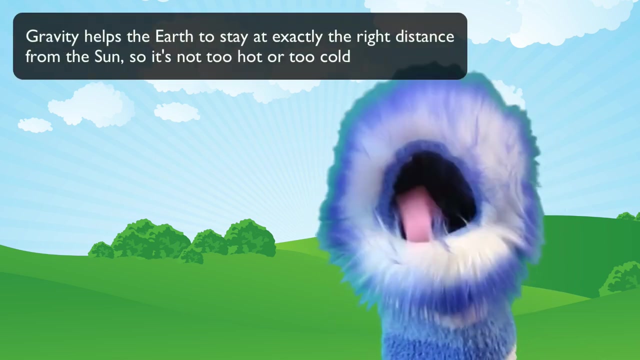 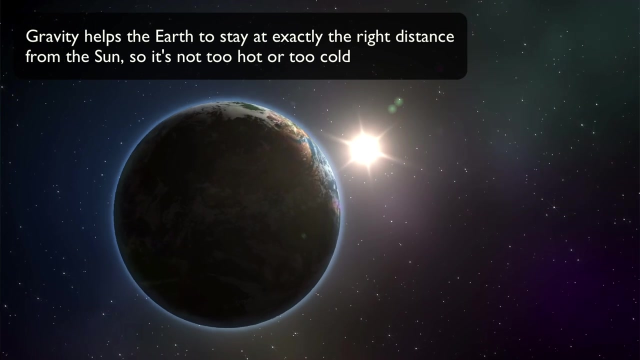 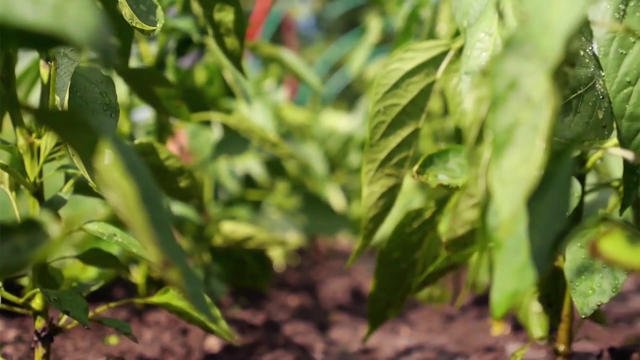 Life on Earth requires the Sun's light, The Sun's light and warmth to survive. Gravity helps the Earth to stay at exactly the right distance from the Sun, so it's not too hot or too cold. Hey, guess what? Gravity even helps guide the way that plants grow.